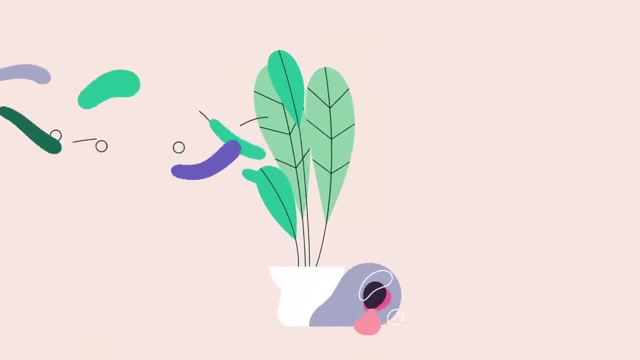 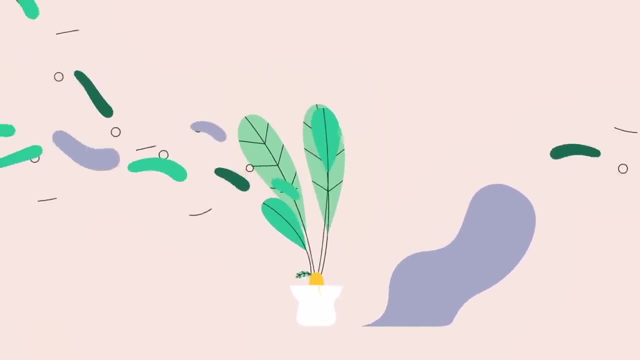 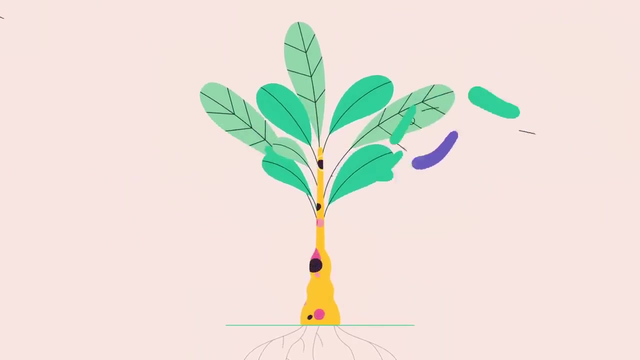 carbohydrates in a reverse process called respiration, converting them to energy and releasing carbon back into the atmosphere. In trees, however, a large portion of that carbon isn't released and instead is stored as newly formed wood tissue During their lifetimes. trees act as carbon vaults. and they continue to draw down carbon for as long as they grow. However, when a tree dies and decays, some of its carbon will be released back into the air. A significant amount of CO2 is stored in the soil, where it can remain for thousands of years, But eventually that carbon also seeps back. 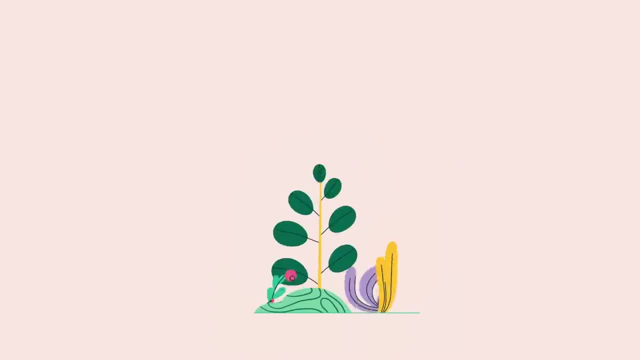 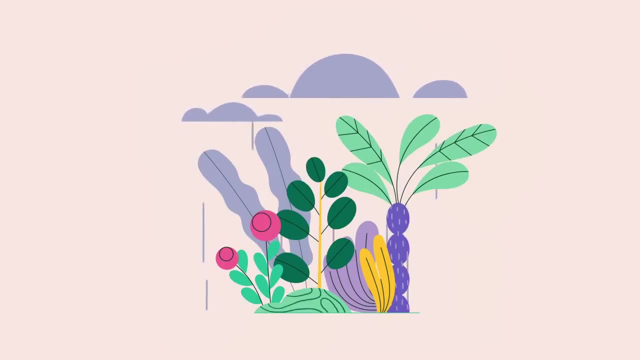 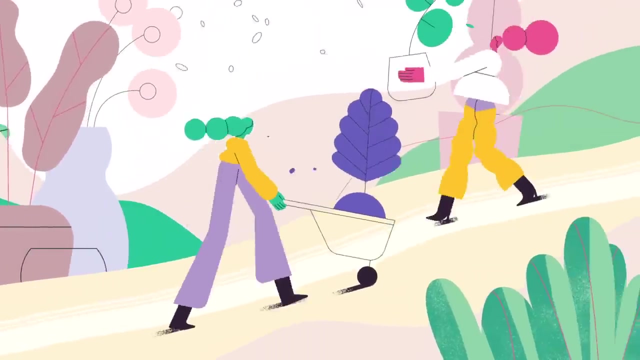 into the atmosphere. So if trees are going to help fight a long-term problem like climate change, they need to survive, to sequester their carbon for the longest period possible, while also reproducing quickly. Is there one type of tree we could plant that meets these criteria? Some fast-growing, long-lived, super-sequestering species we could scatter worldwide- Not that we know of. But even if such a tree existed, it wouldn't be a good long-term solution. Forests are complex networks of living organisms and there's no one species. 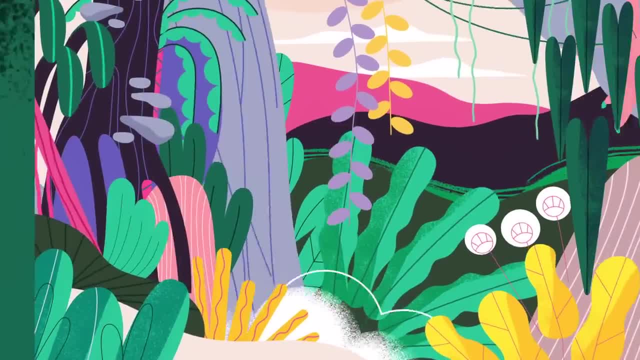 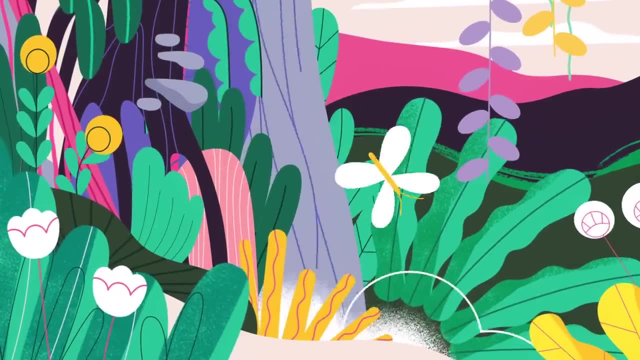 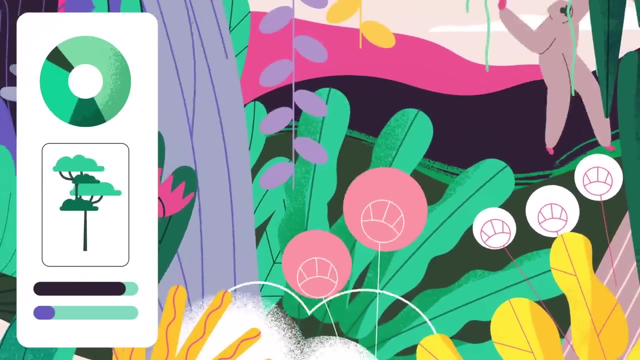 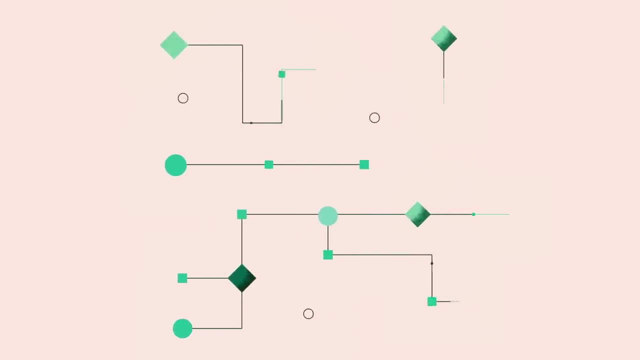 that can thrive in every ecosystem. The most sustainable trees to plant are always native ones, species that already play a role in their local environment. Preliminary research shows that ecosystems with a naturally occurring diversity of trees have less competition for resources and better resist climate change. This means we can't just plant trees to draw down carbon. 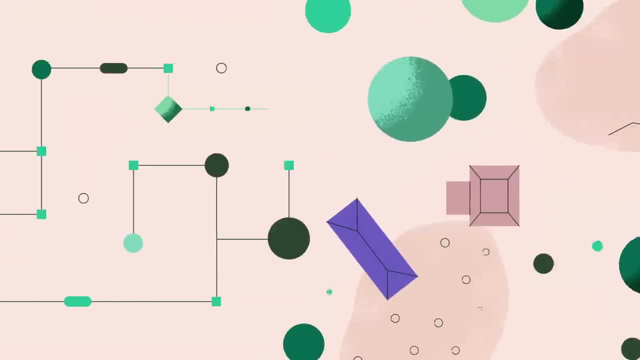 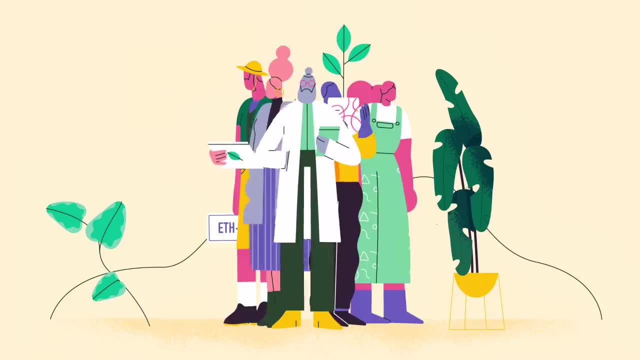 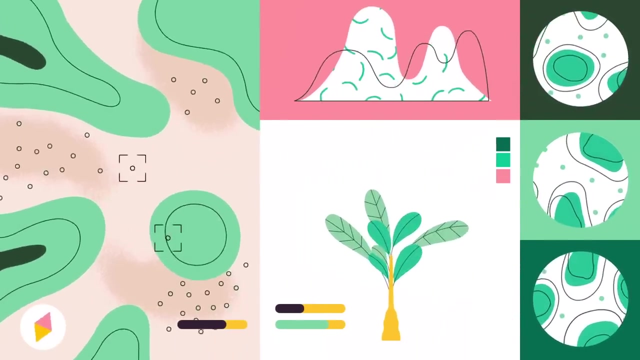 We need to restore depleted ecosystems. There are numerous regions that have been clear-cut or developed that are ripe for restoring In 2019,. a study led by Zurich's Crowther Lab analyzed satellite imagery of the world's existing tree cover By combining it with climate and soil data and excluding areas. necessary for human use. they determined Earth could support nearly 1 billion hectares of additional forest, That's roughly 1.2 trillion trees. This staggering number surprised the scientific community, prompting additional research. Scientists now cite a more conservative but still remarkable figure By their revised estimates. 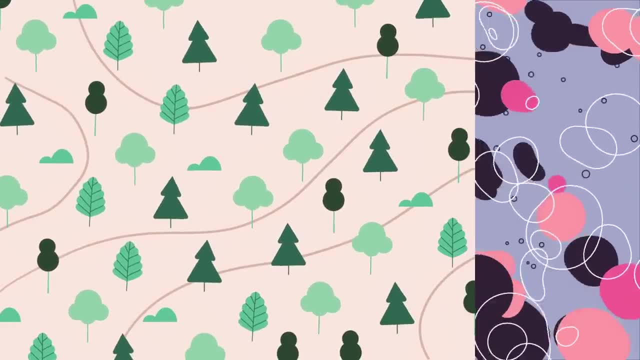 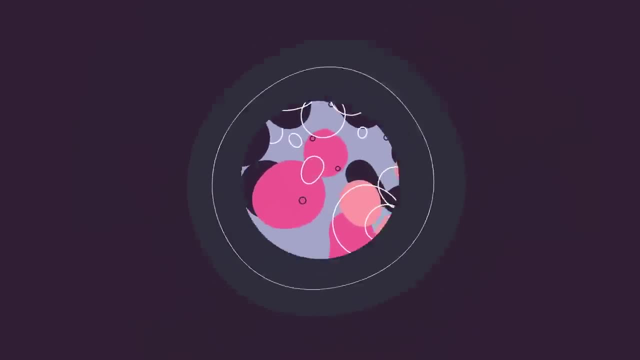 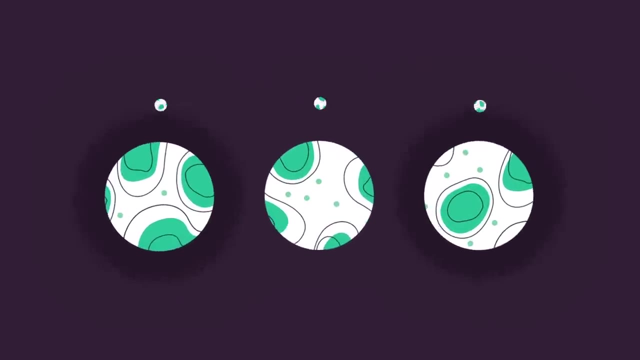 these restored ecosystems could capture anywhere from 100 to 200 billion tons of carbon, accounting for over one-sixth of humanity's carbon emissions. More than half of the potential forest canopy for new restoration efforts can be found in just six countries, And the study can also provide insight into existing 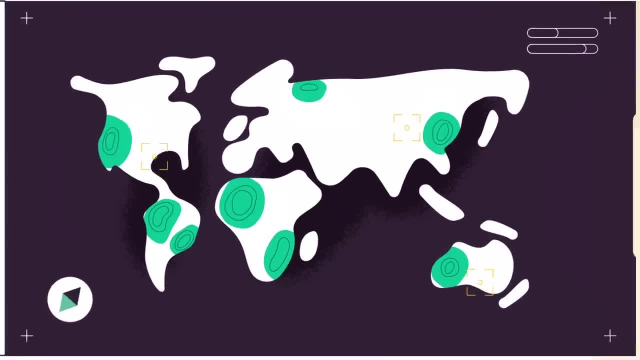 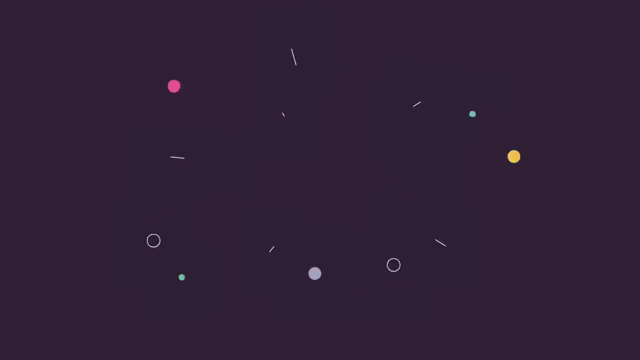 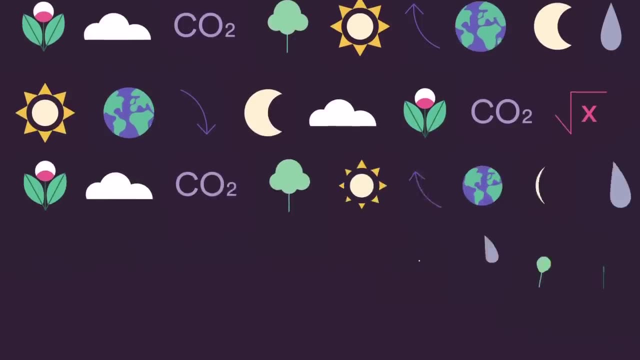 restoration projects like the Bonn Challenge, which aims to restore 350 million hectares of forest by 2030.. But this is where it gets complicated. Ecosystems are incredibly complex and it's unclear whether they're best restored by human intervention.